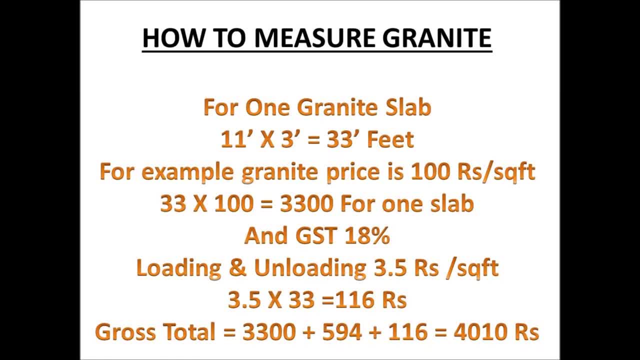 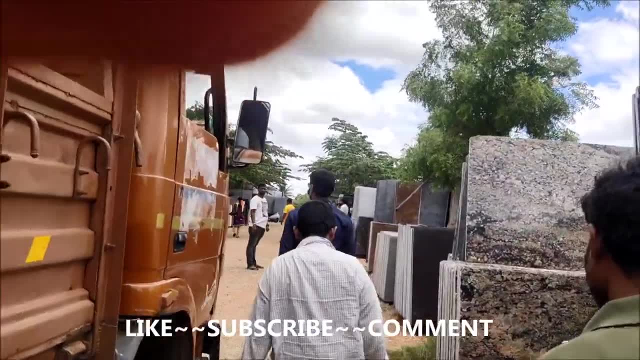 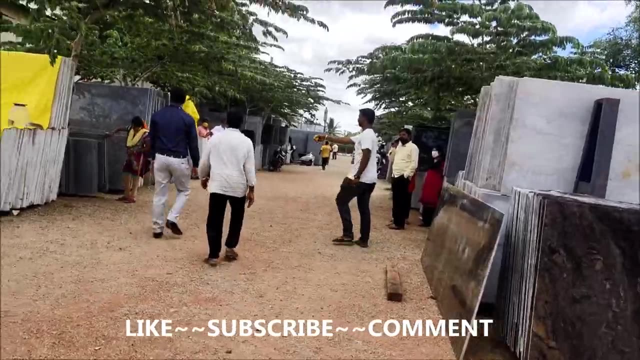 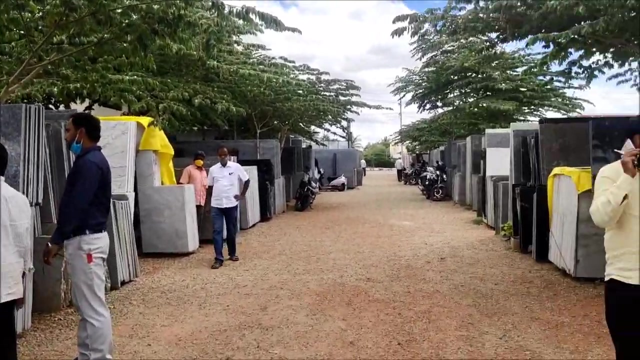 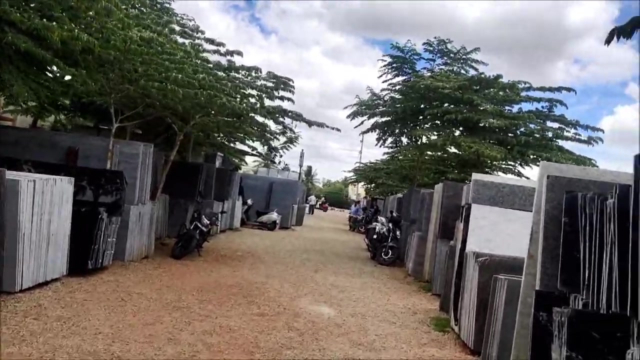 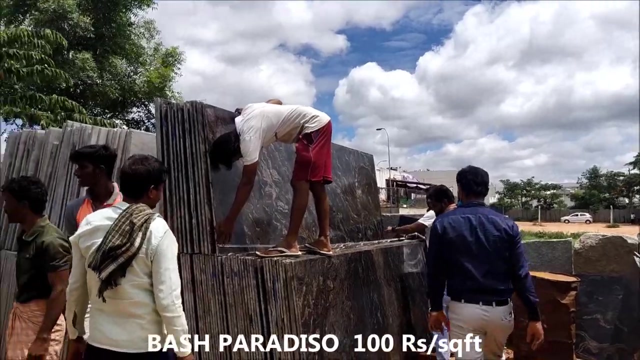 In the next video, I will show you the different types of granites: colors, price and rates. Okay, So let's get started. So I've got. so I've got a special type of granite slab. This one is called a granite slab. This one is called a granite slab. 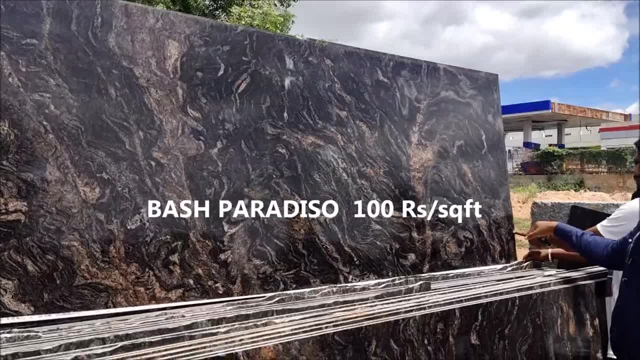 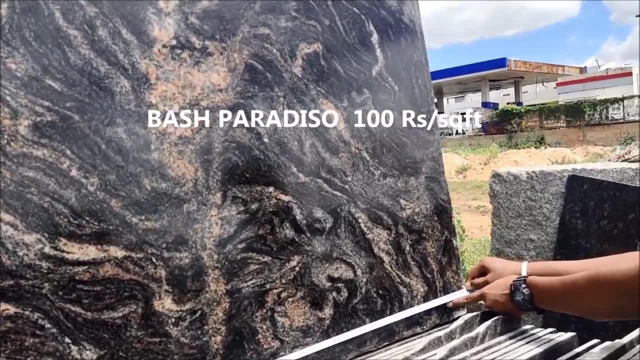 It is a very bad kind of granite slab. The problem is that you have to buy it and you have to buy a lot of different types of granite. For example, the answer is infections. So there is a problem in this type of granite slab and its weight is very high. 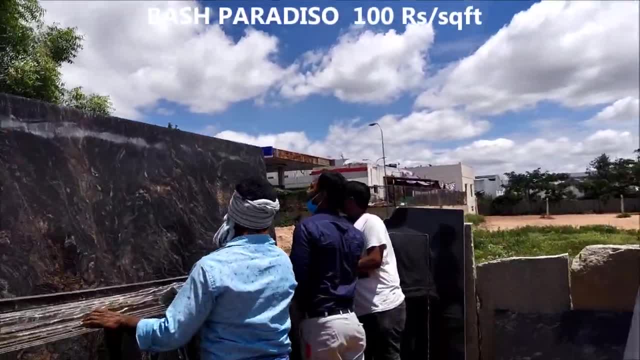 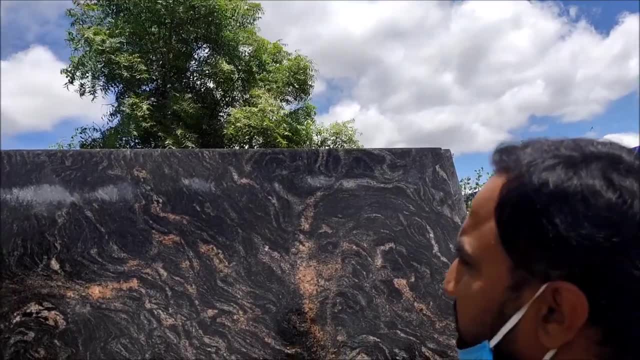 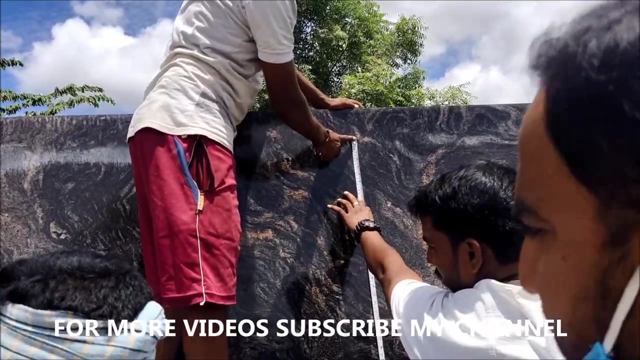 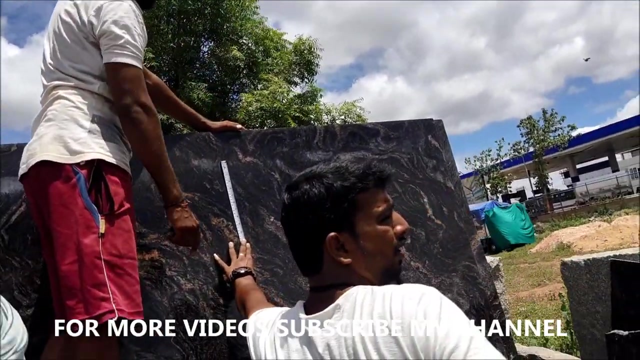 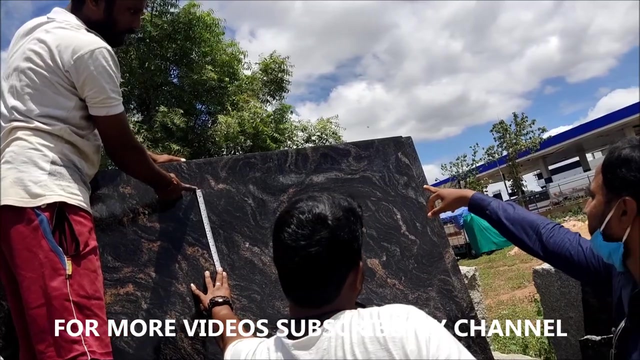 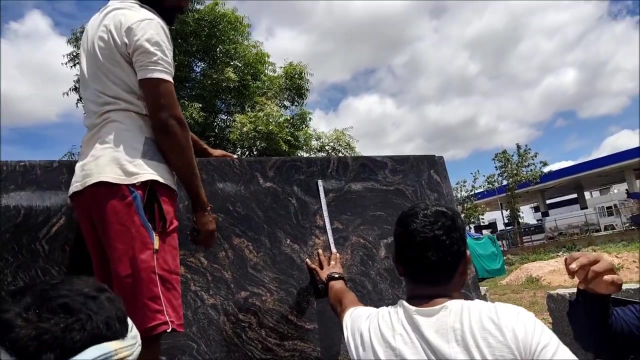 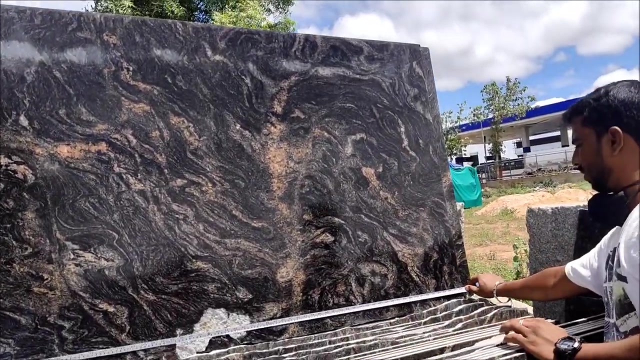 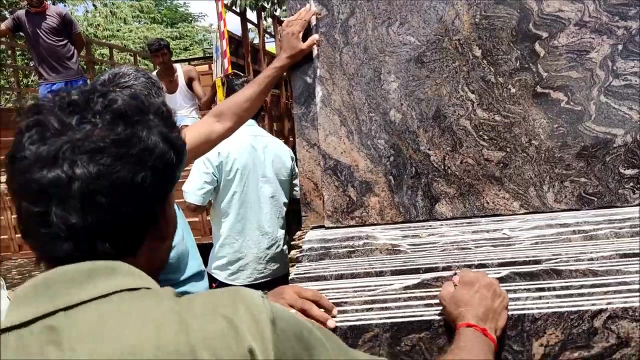 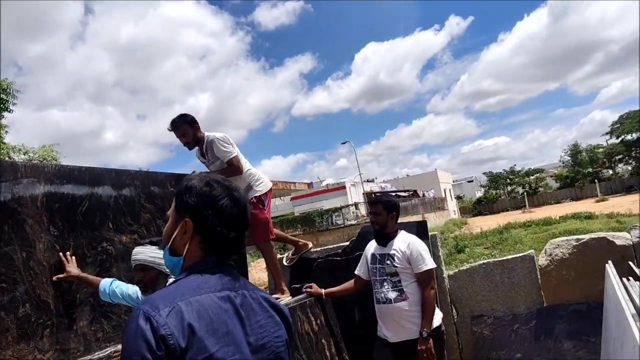 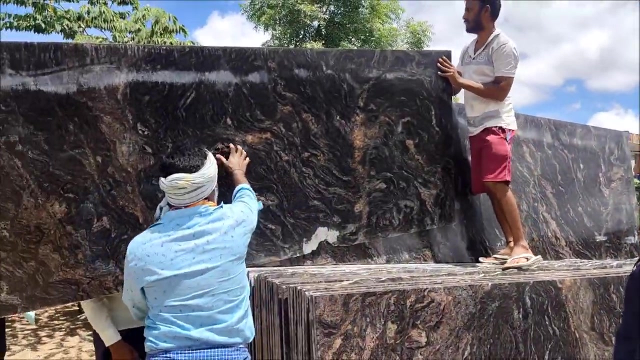 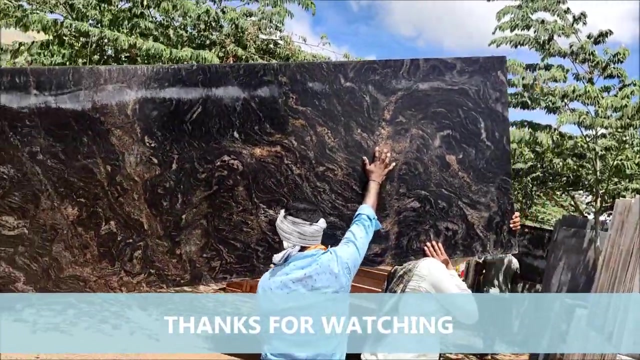 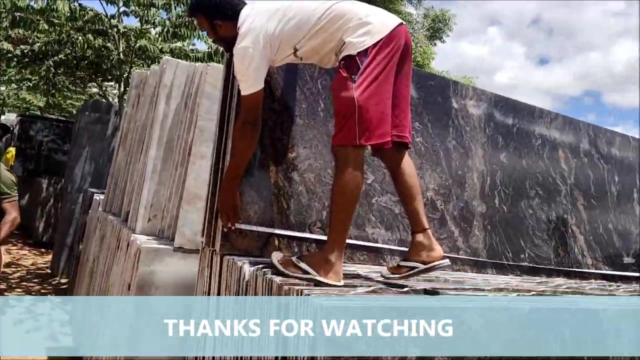 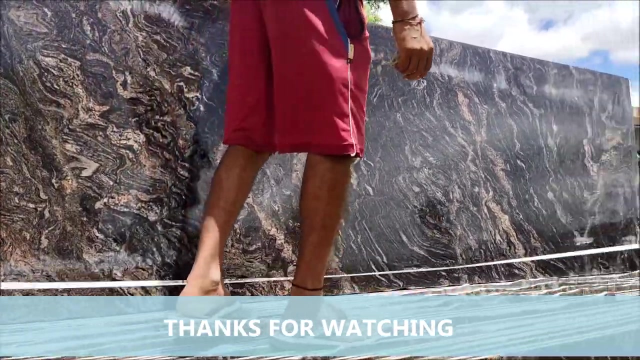 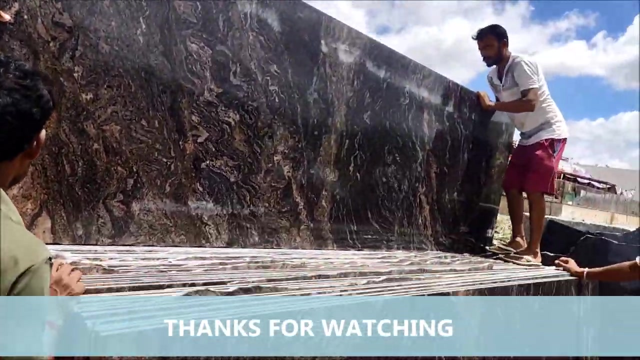 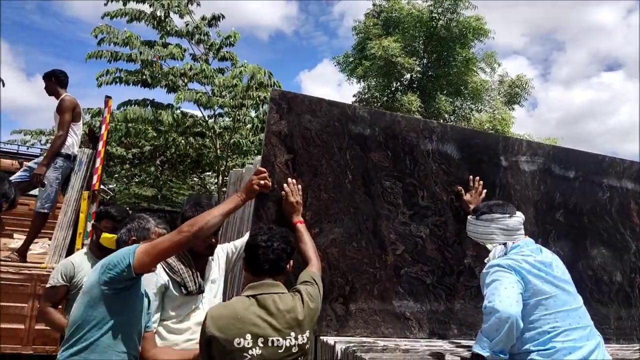 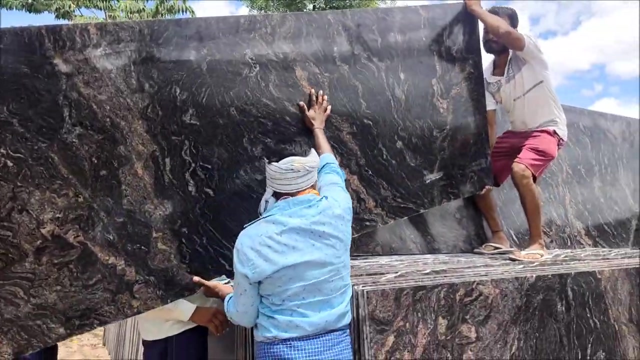 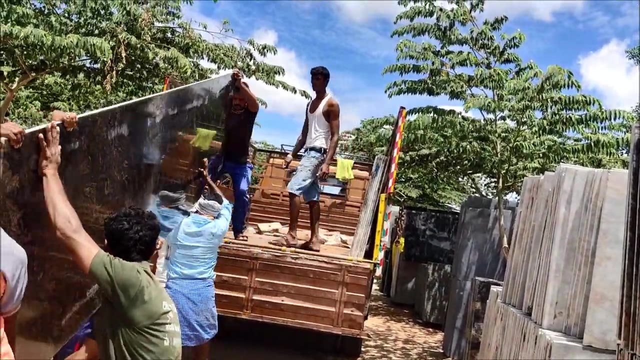